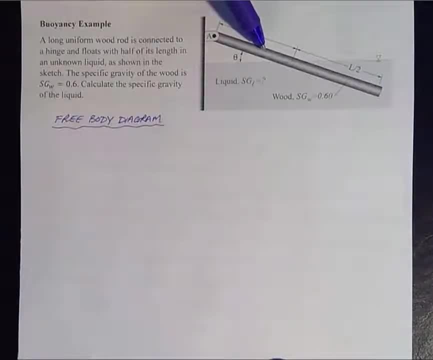 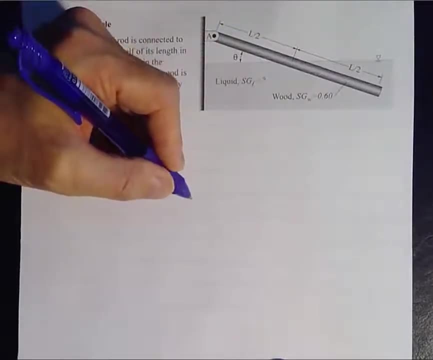 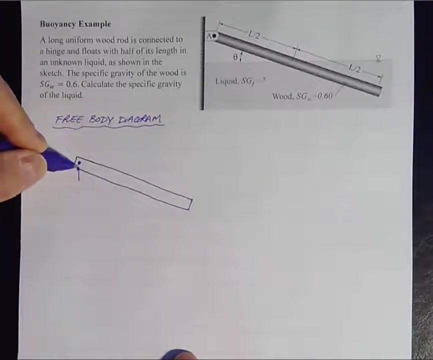 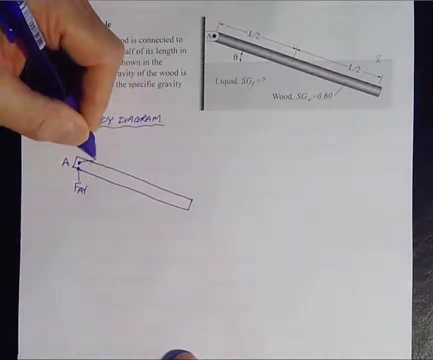 diagram itself over here. you want to draw this rod floating in the air And put all the forces on it, So I'll do that. Here's point A, that's the hinge, And don't forget there's forces at the hinge. So I'll call that F? A in the y direction, F? A in the. 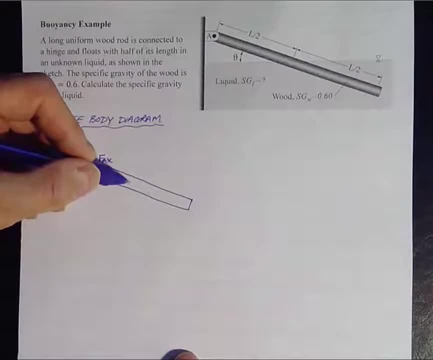 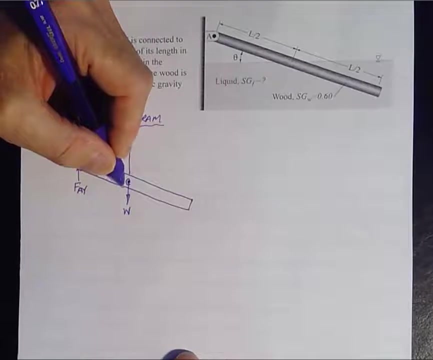 x direction. Now, the forces you have, of course, acting at the center is a long, uniform, long rod. right at the dead center of this rod, right at it's centroid, it would have it's weight and it would act at, of course, this distance here, If the rod is inclined at an 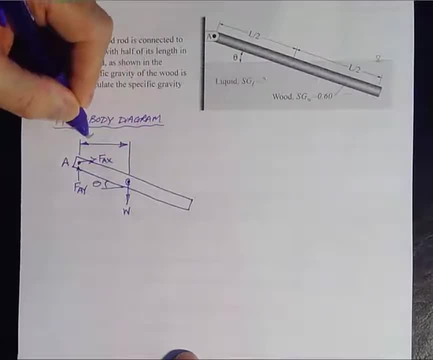 angle theta, then this distance here is clearly L upon two cos theta. Now the buoyancy force, which is- this is known as coalesce force, and that's the angle that's going to actually form the coalesce of the rod And it's going to be coalesce over here. This angle is going. 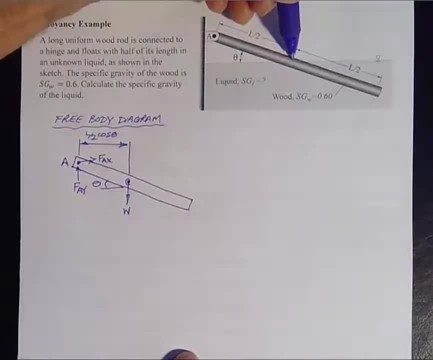 to form the coalesce of the rod And we're going to go over and see if that's accurate, acts at the center of the displaced volume. So half of this rod here is below the water, So it's going to act at the center of this place volume which would be right there Upwards. 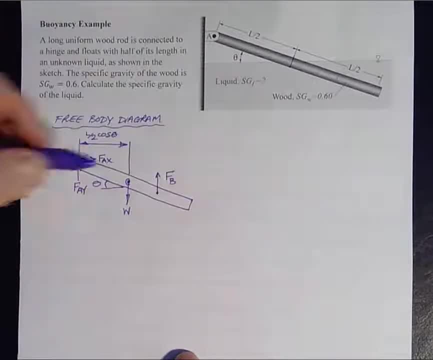 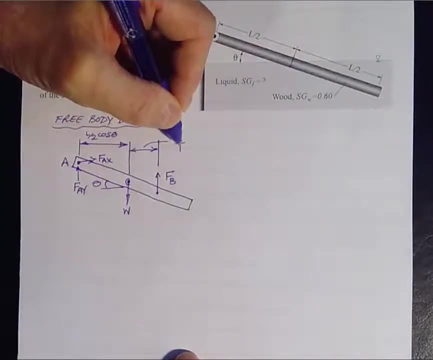 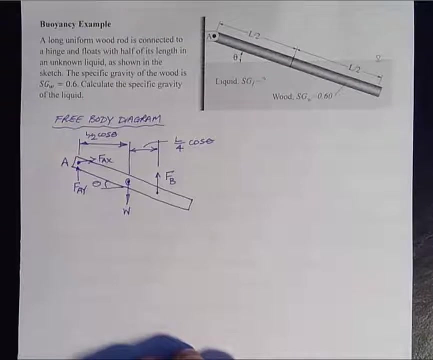 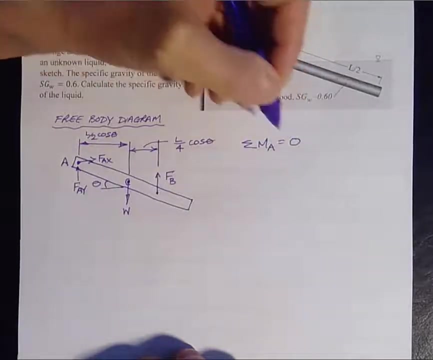 here's the buoyancy force, And this distance here is going to be L upon four goes theta. So that completes our free body diagram. So what we do is we take some of the moments about the hinge equal to zero. we take the moments around the hinge, of course. 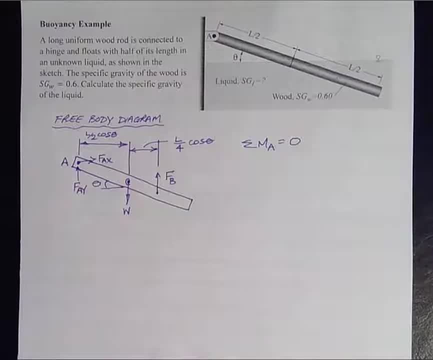 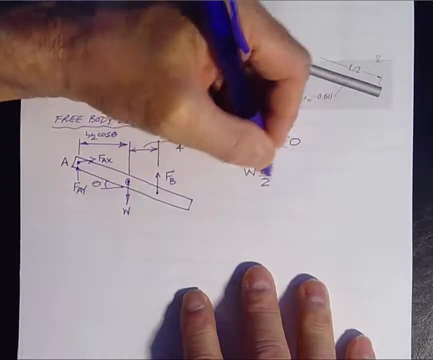 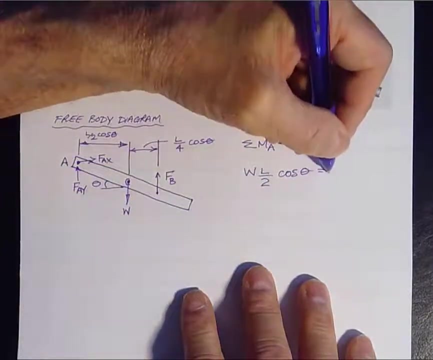 so that we don't have to calculate the hinge forces, And so we would have that W? L upon two cos theta. so it's the weight times. the moment arm has got to equal the buoyancy force times. its moment arm, which you can see is three quarters L cos. 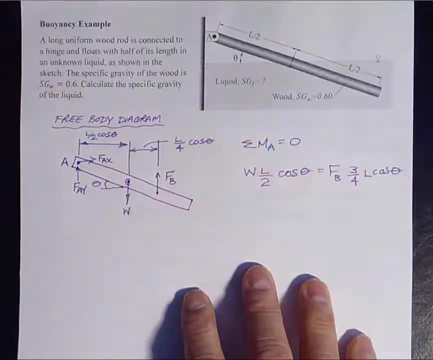 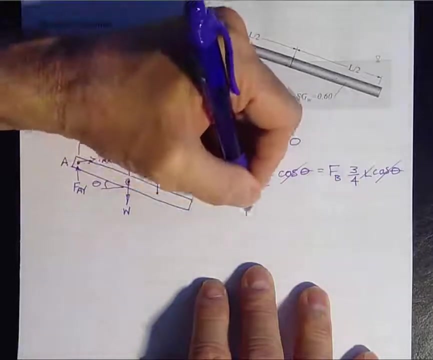 theta. So now we can see that the L cos thetas cancel out. It really doesn't matter. That's why we weren't told the angle in this problem. It's independent of the angle And we get that the buoyancy force in static equilibrium is two thirds of. 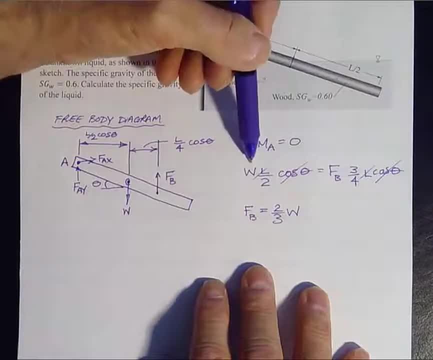 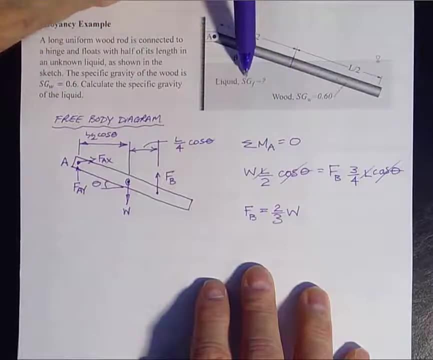 the angle And we get that the buoyancy force in static equilibrium is two thirds of the weight. So now we need to figure out what the weight and the buoyancy force terms are in terms of the specific gravity of the unknown fluid and the wood. So the weight is pretty straightforward. 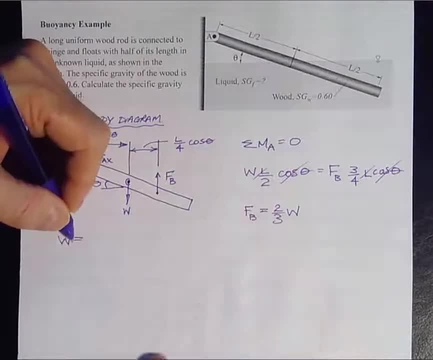 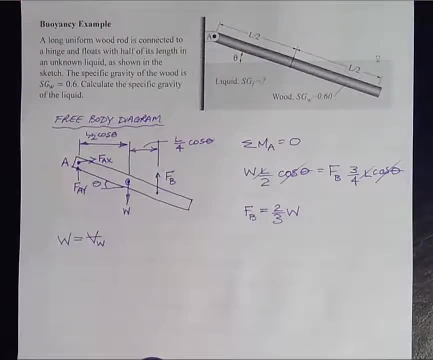 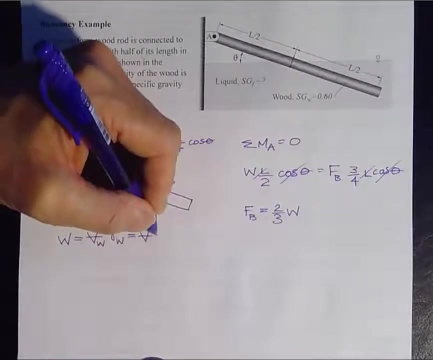 Let's do that first. The weight of the wood is just the volume of the wood, whatever. the total volume of the wood is times the gamma of the wood. I'm going to put that in terms of specific gravity, So that would be equal to the volume of the wood. specific gravity of the 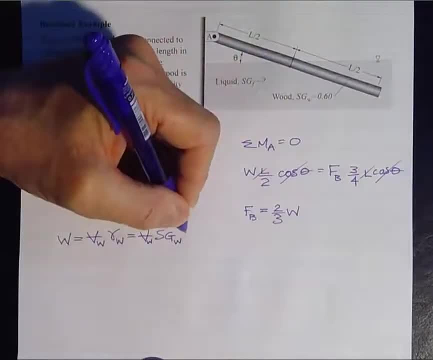 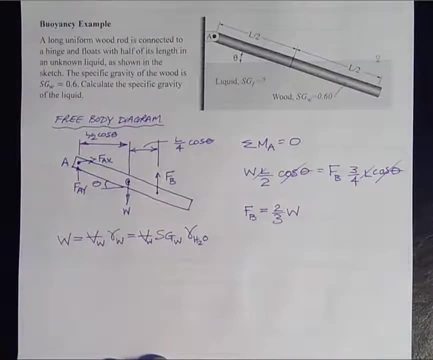 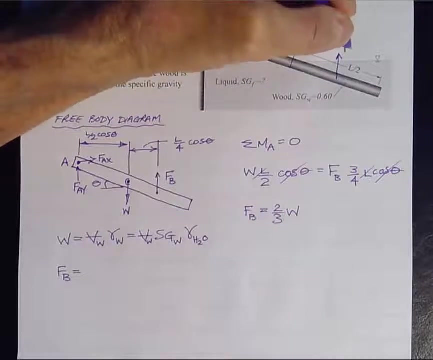 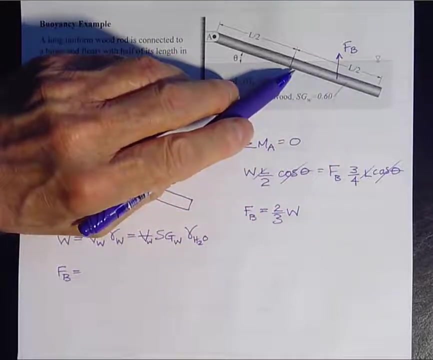 wood which we know is point six times the gamma of water, technically at four degrees C. Now the buoyancy force. this is perhaps the crux of the problem. The buoyancy force acts at the center of the displaced volume here right And half of the rod is below the water line And it's equal to the 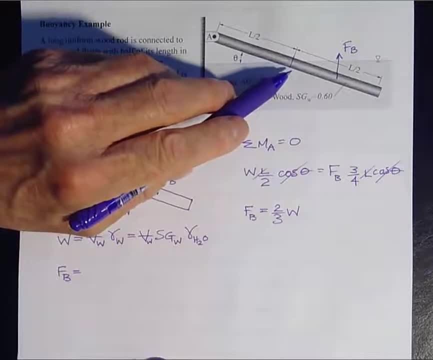 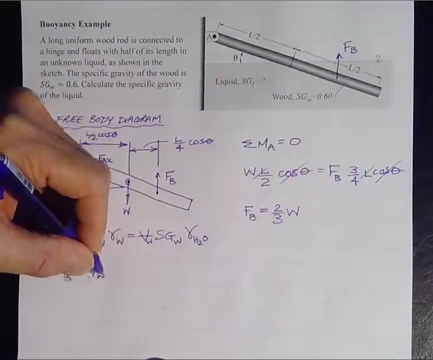 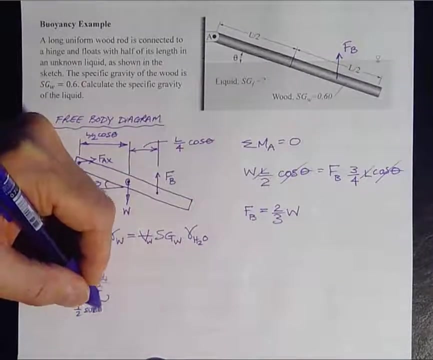 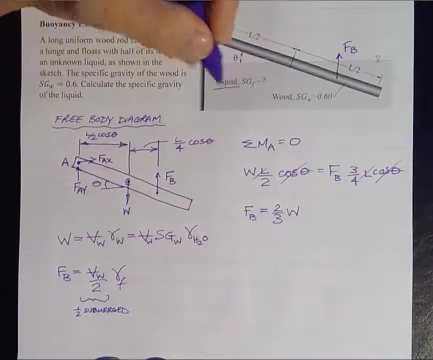 weight of the displaced fluid, of the unknown displaced fluid. So it's going to be half of the volume of the wood. Make a little note here: this is because we're one half submerged times the gamma, the specific weight of the unknown liquid here. So we can put that now in terms of the specific 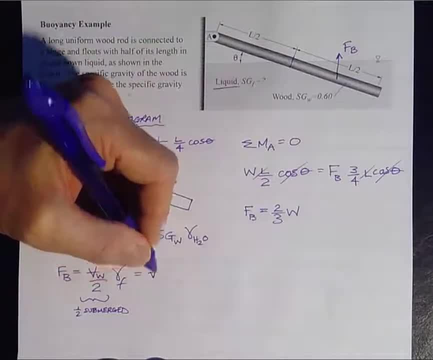 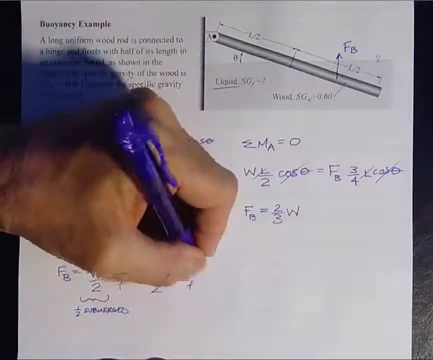 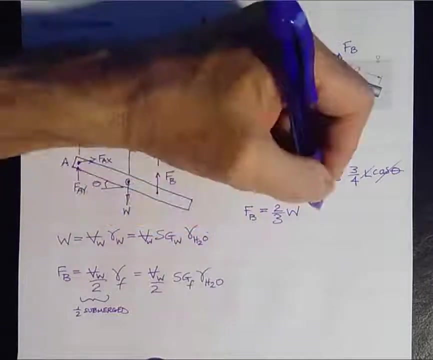 gravity of the unknown liquid. So that'll be volume of wood divided by two. specific gravity of the fluid, which is what we're after, times the gamma of water at four degrees C. Okay, let's okay. we'll call this equation one. we'll call this equation two. we'll call this equation.